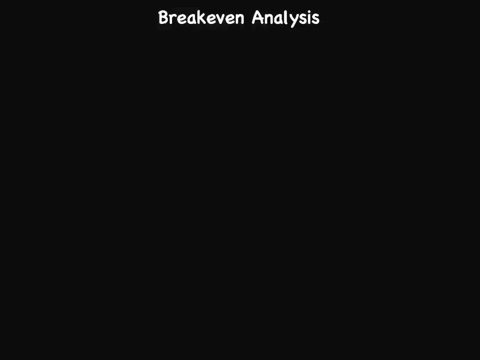 fine-tuning the actual pricing. Businesses have to consider a lot of different things if they're going to price their products not only competitively, but also to the point where they're going to cover a lot of their costs, And so one of the easiest ways or easiest tools that you can 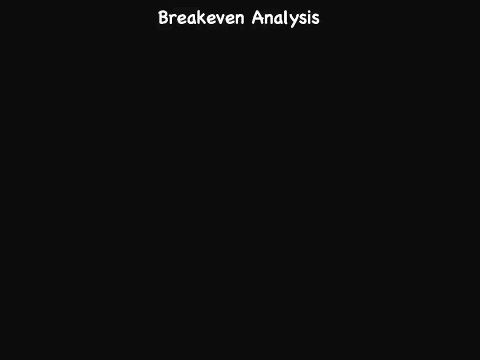 utilize is what we call a break-even analysis, And a break-even analysis is simply a process that's used to determine the number of units that you would have to sell to cover your cost, And so I'll abbreviate the break-even point as BP, And so we're going to refer to the number of units. 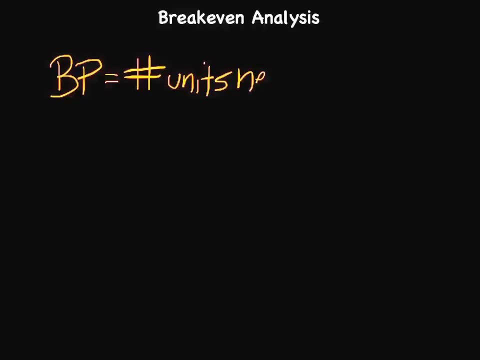 that are needed to cover your cost, To cover our costs, And so ideally, as a business, you wouldn't just sell whatever number. this is because you're covering your cost. You're not necessarily making any money. Ideally, you'd be able to sell more than this, And so this is a great starting point for a discussion: to know that. 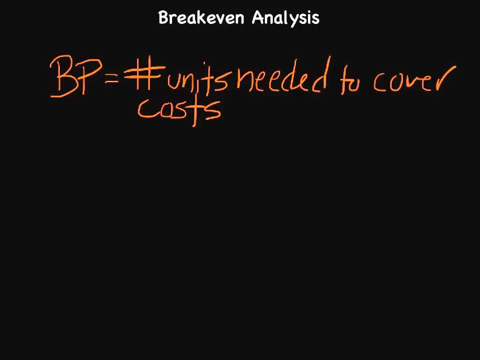 well, is it feasible for us to sell this number of products? And if it is great. If it isn't, though, well, what are some of the things that we can do? What are the variables that we can change so that it is a little more reasonable? So let's go through. Let me show you first. 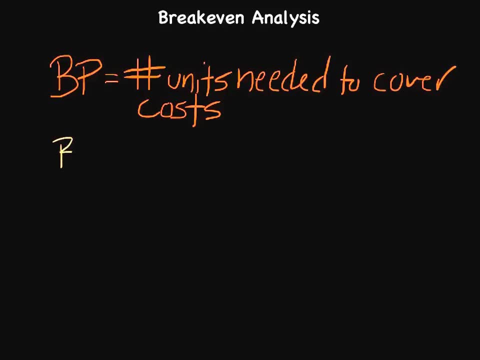 what the equation is for a break-even point. And the break-even point is simply: first, your fixed costs. Fixed costs do not vary over time within a certain relevant range, And so these often include things like plants and property and equipment, and even advertising insurance taxes. These are 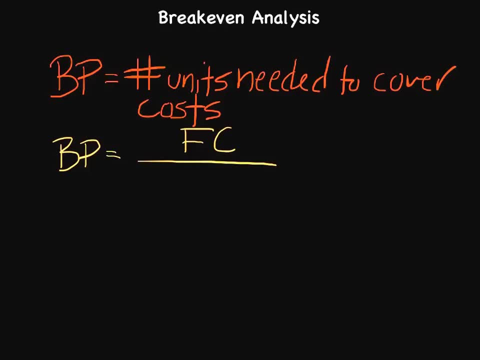 commonly fixed costs. And the reason they're fixed is because they're not just fixed costs, They're based upon the number of products that you sell. So if I sell nothing, I know I still have to pay utilities. I still have to pay the lease for the property I'm using. I still have to pay certain 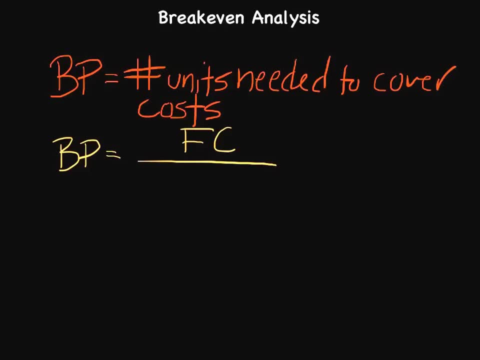 insurance costs and different things. I still pay advertising And so they're fixed. They don't vary based upon production. So I take my fixed costs And then what I do, as I divide that by first my price of my product. So whatever is the selling price for my product, what consumers have? 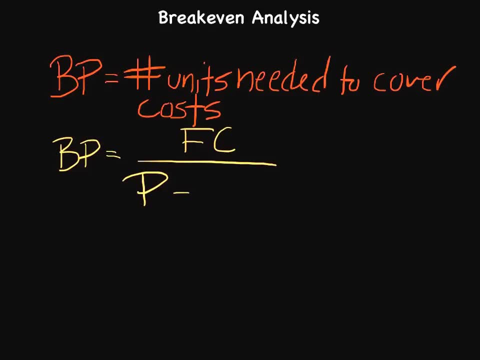 to give up to obtain my product less what we call variable costs, which I'll abbreviate as VC. And variable costs, contrary to fixed costs, vary based upon the number of units produced, And so if you produce you know five of a particular product, then ultimately you're. 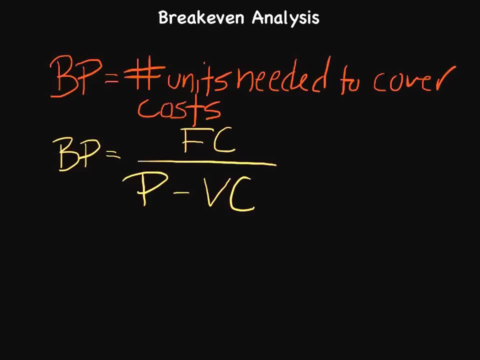 going to take your fixed costs multiplied by five, So they go up with every unit they're produced. Typically, variable costs include things like direct materials, And so the materials that actually went into the product are the ones that are produced, And so the materials that are 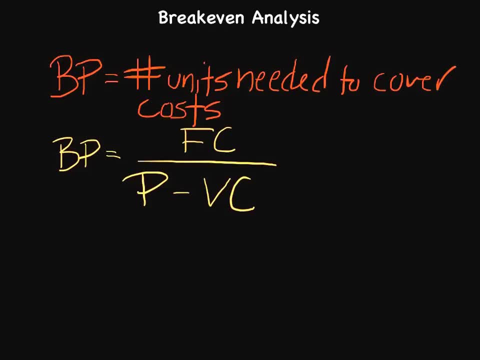 assembled into. assembling that product typically includes direct labor, And so the actual people that assembled the product and that put it together- obviously, the more time they spent is based upon how much you produce. So those are all things that you would essentially consider in variable costs, and then a few other things. So let me show you how you would actually work. 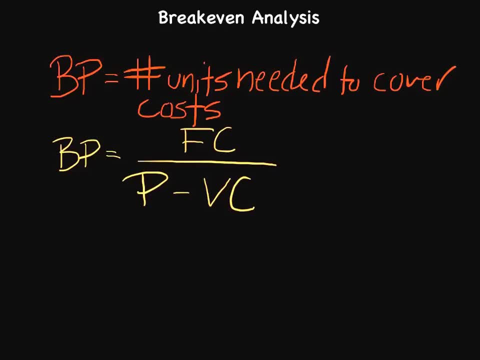 this here. Let's say that we actually produce cell phone cases and we have a fixed cost of $500,000.. And so these are the costs that we incur, just without any production whatsoever. This is plants, property, equipment, advertising taxes. those types of things do not vary based upon how many. 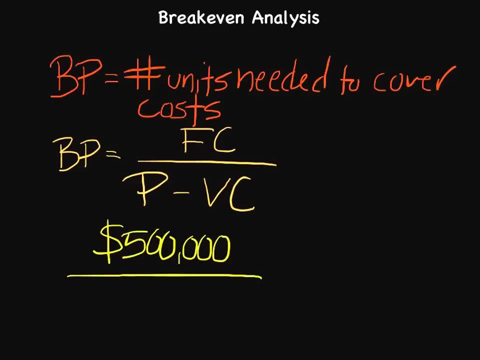 units we sell, And we sell these cell phone cases for, let's just say, $20 each And it costs us about $10 in fixed costs to make them. So for every case we can sell for $20, we pay $10 to. 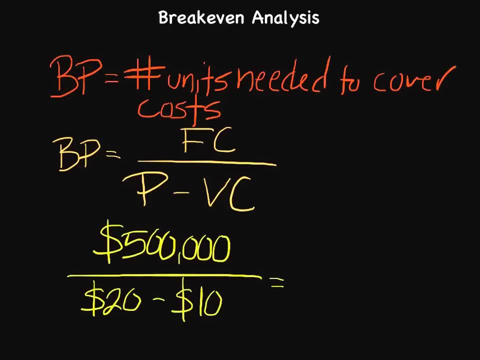 actually have it made. So with this equation we would actually have a fixed cost of $20.. And so we have a break-even point of 50,000 units. And so whether or not this is attractive will depend on a number of different factors. You may look at this and say: I have to produce. 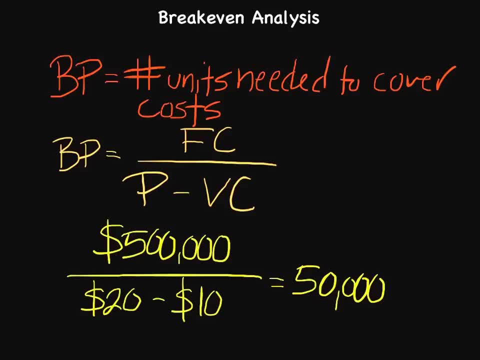 50,000, or sell- not produce, but sell- 50,000 of these cases in order for me just to cover the costs that I have, And in large part that's driven by the fixed costs, which are a little high. But that might not be feasible, right? Or it may be well, 50,000, that's nothing I was. 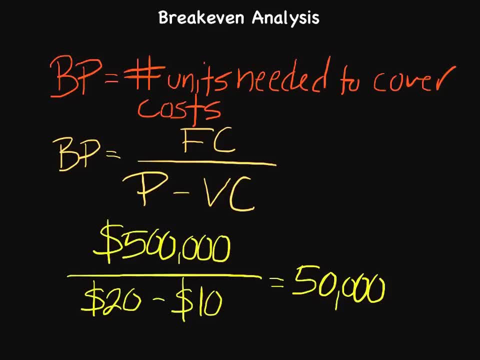 going to sell way more than that, or I'm projected to sell a lot of these cases, So I'm going to sell a lot more than that. In that case, this might be very encouraging, But if it's not, if this is, 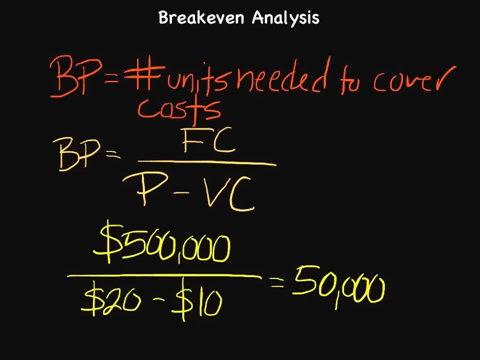 somewhat of a concern, right, If you're planning well. I thought I was going to sell about 5,000 the first year, not 50,000.. I don't want to be in the negative for an extended period of time. 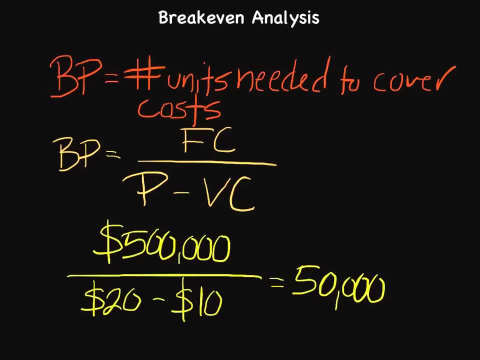 That doesn't necessarily mean that you should just scrap everything and go back to the drawing board. This is a starting point for a good discussion, And the reason is is that you might be able to change a couple of these variables. right, There are three variables. 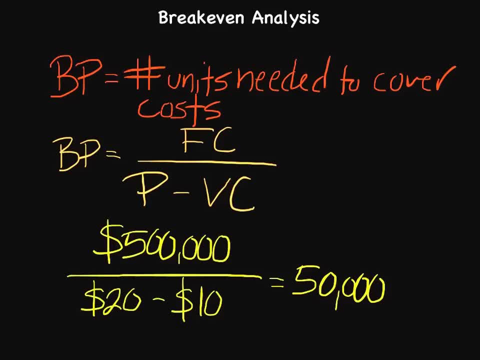 that are here- fixed costs, price and variable costs- And so maybe we can actually change things right. We can do a couple of different things. Maybe we have the ability to raise our price a little bit. Maybe we're not priced competitively. 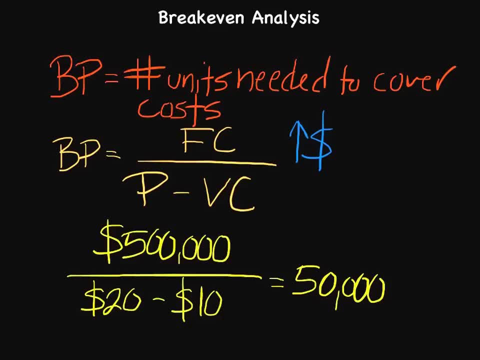 We're undercutting ourselves, And so if we raise price, that means our margins are better, which in turn means we don't need to sell as many products to actually break even. right, The break even point would be less than 50,000 units, So that's one thing we can look at. 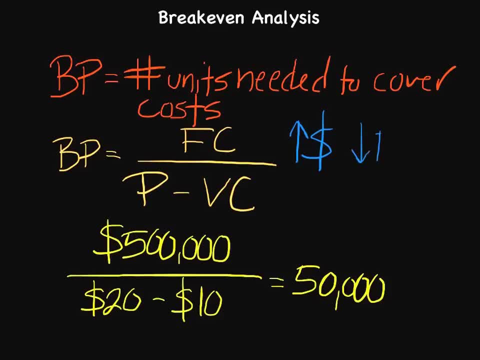 We can look at possibly reducing our fixed costs. right. Things like the actual plant that we're using, right? Maybe it's too big for us. Maybe we can actually downsize, get a smaller plant still be able to produce effectively and efficiently. 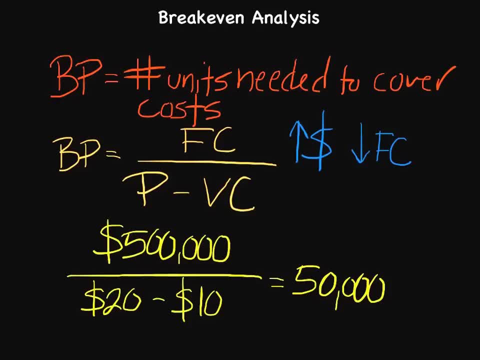 but now we're lowering our fixed costs. Maybe we need to reduce our advertising expenditures, Maybe we need to reduce, you know, the utilities that we pay, which would be kind of similar to, you know, reducing our plant size. We probably wouldn't pay as much in utilities, And so 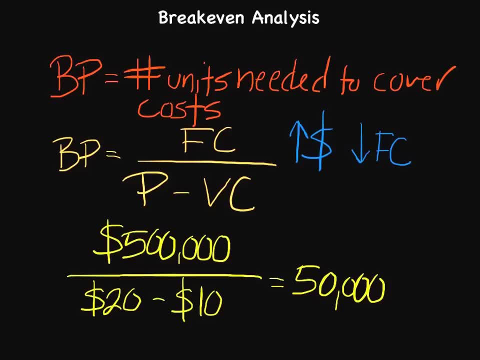 if you lower your fixed costs, that would also make it so that you wouldn't need to sell as many products to just reduce your fixed costs. So that's one thing we can look at, And the other thing we can look at is just break even And then, lastly, we can lower those variable costs. 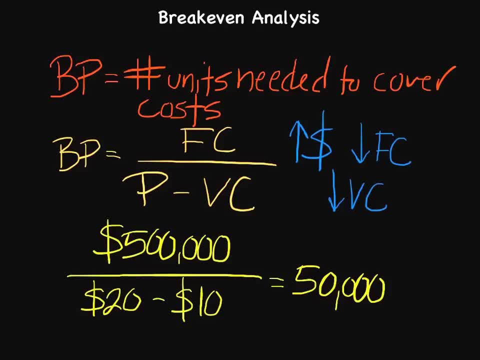 right The costs that are directly associated with producing products, And so this can include finding maybe less expensive materials to go into the product. Obviously, try not to sacrifice quality to any significant degree. We can try and find more efficient ways of producing the product. 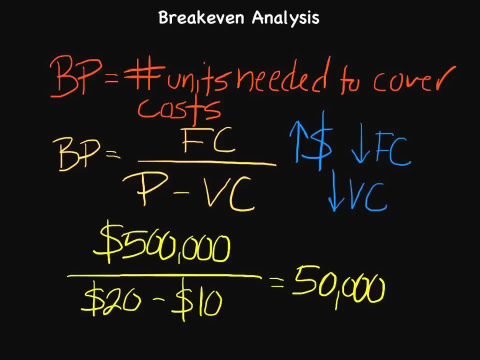 So maybe we don't have to pay as much in labor to produce them. We find cheaper ways to do that, maybe faster ways to do that, And so those are some things that you can consider: Raising prices, decreasing variable costs, decreasing fixed costs, The